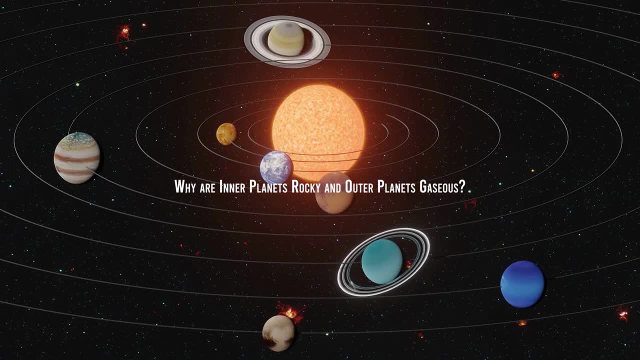 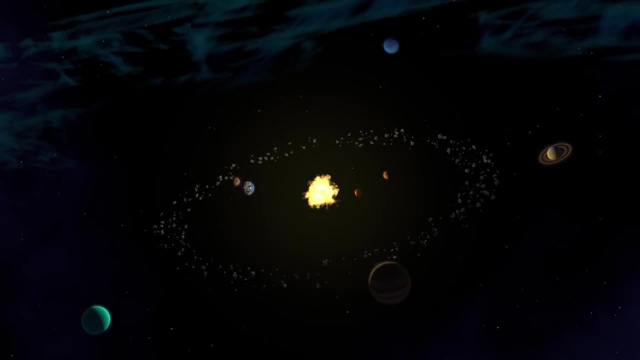 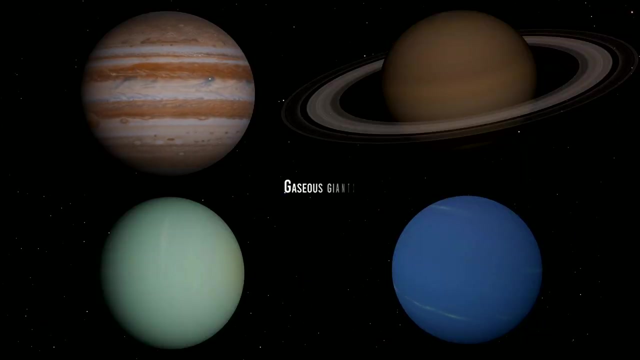 Why are inner planets rocky and outer planets gaseous? We all know the solar system contains two kinds of planets. The first four, Mercury through Mars, are quite small in size and they are rocky planets, also called terrestrial planets. The outer four are gaseous giants, from Jupiter to Neptune. They are called Jovian planets. 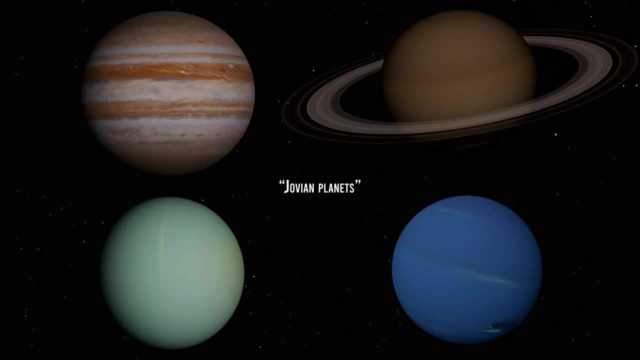 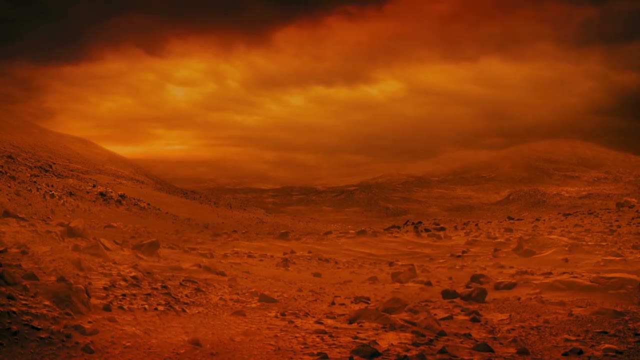 and they are immense balls of gas with a central core. While conditions on these planets can be very different from one another, each type of planet shares some similarities and offers its own set of challenges when it comes to exploration and observation. But where does this difference come from? 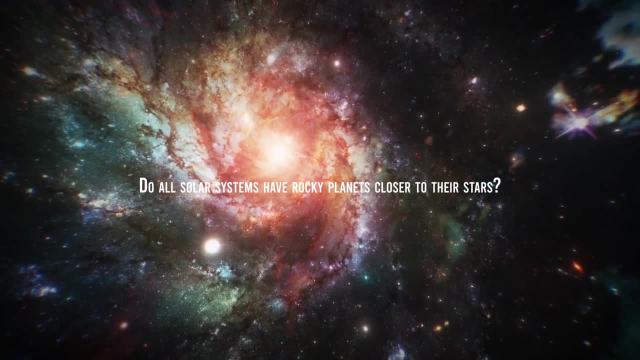 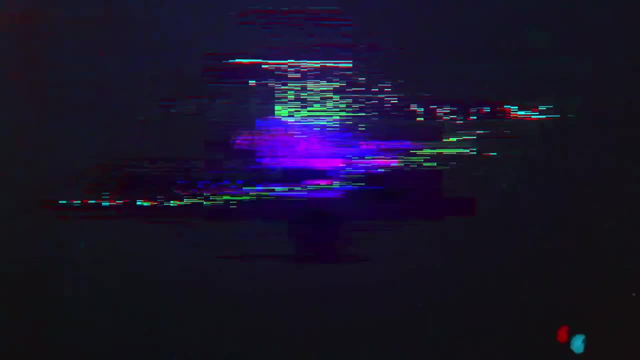 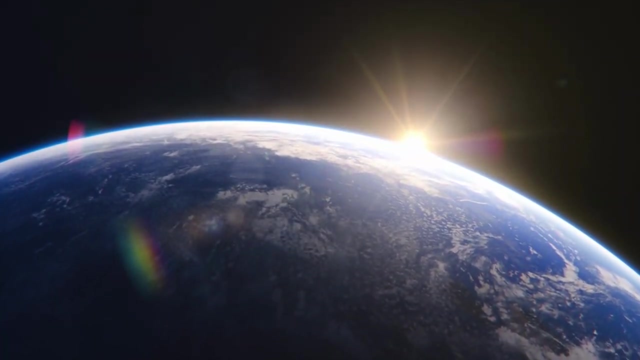 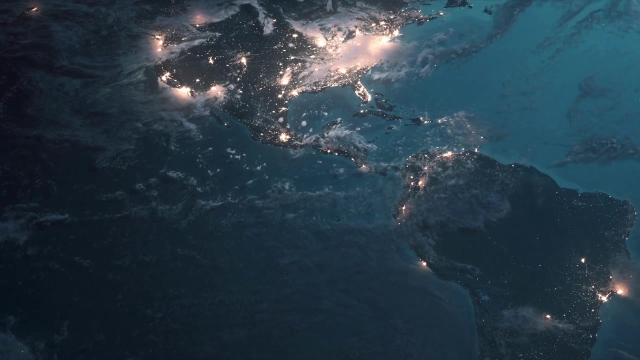 Do all solar systems have rocky planets closer to their stars? Keep watching the video to get to know the answer to these questions, and more. The Earth is perhaps the most important rocky planet in our solar system. On Earth, the core, mantle and crust, are divisions based on compositions. 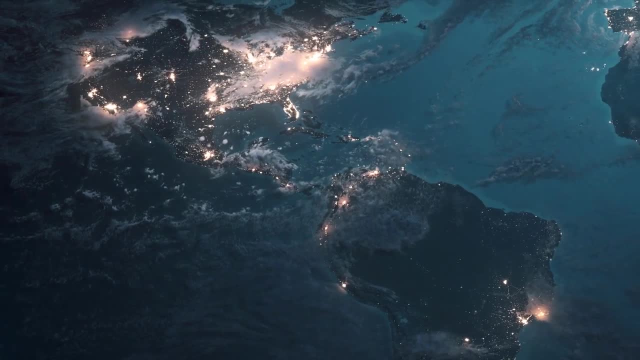 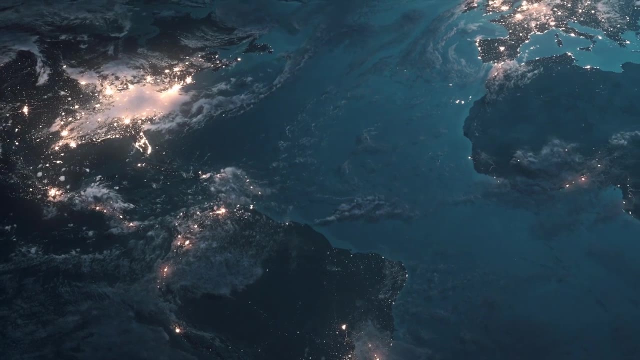 The crust is really a small part of the overall Earth's mass, accounting for less than 1%. It consists of oceanic crust and continental crust is often more felsic rock. The crust is where we live, the place we walk on and the most exposed layer of our planet. 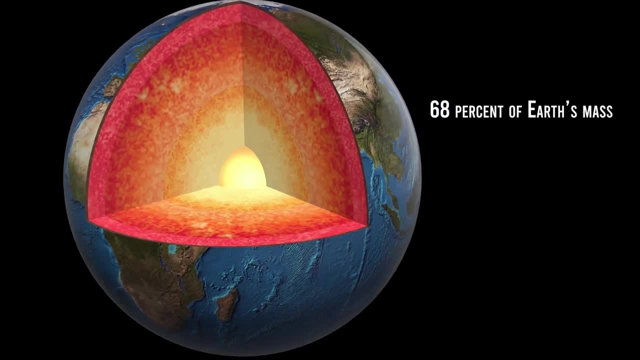 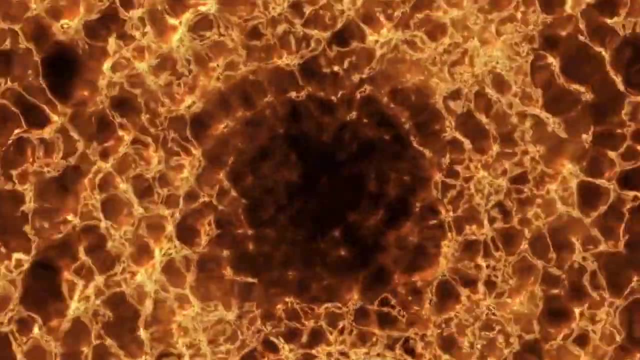 Then there is the mantle. The mantle is hot and represents about 68% of Earth's mass, And if you go deeper you can reach the core. I mean, you can't really, because the deeper you go, the stronger the pressure. 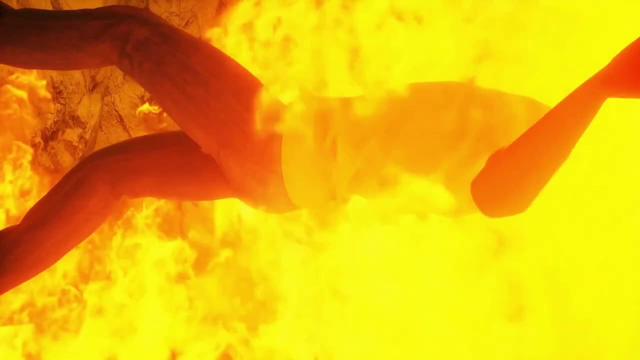 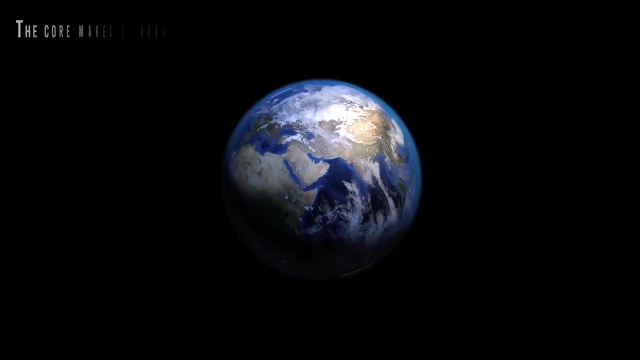 and you'll reach a point where you won't be able to survive anymore. But let's suppose this doesn't happen. If you could reach the core, you would see it's made of iron metal. The core makes up about 31% of the Earth. One may ask: how do we know the core? 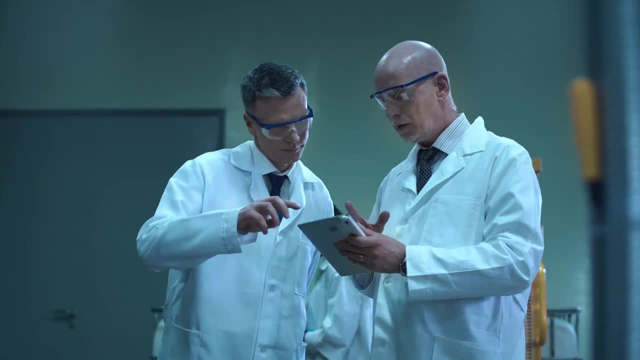 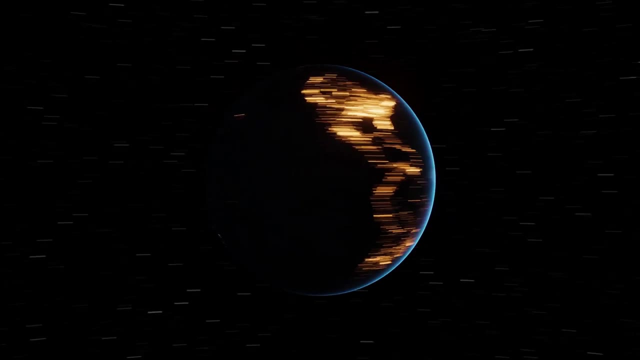 is metallic. Scientists know that the core is metal for a few reasons. First of all, the rotation of Earth gives us some hints about the average density of our planet. It can be shown that the average density given by the rotation is much more than the density of Earth's surface layers. 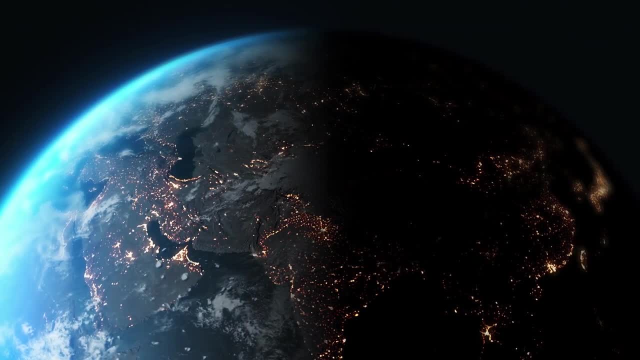 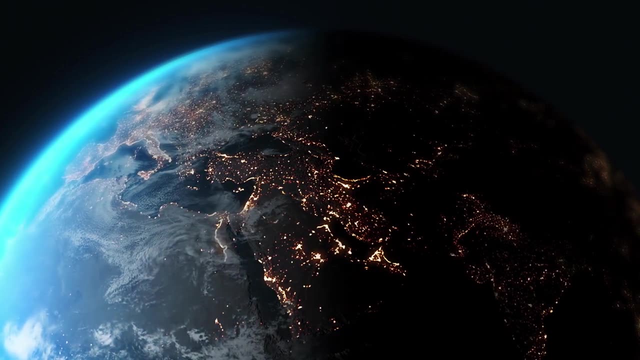 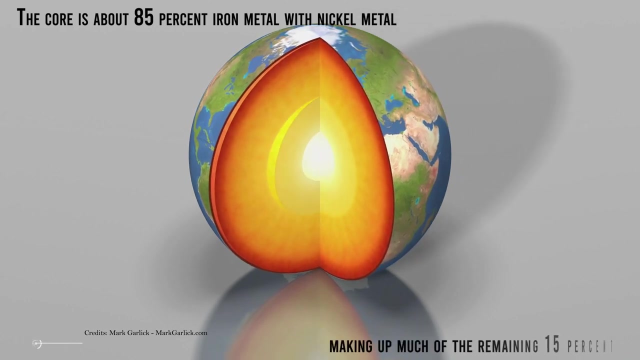 which we can measure. The only way for this to happen is to have an interior denser than the average. Basically, if surface layers are less dense than average, then the interior must be denser than average. Calculations indicate that the core is about 85% iron metal with nickel. 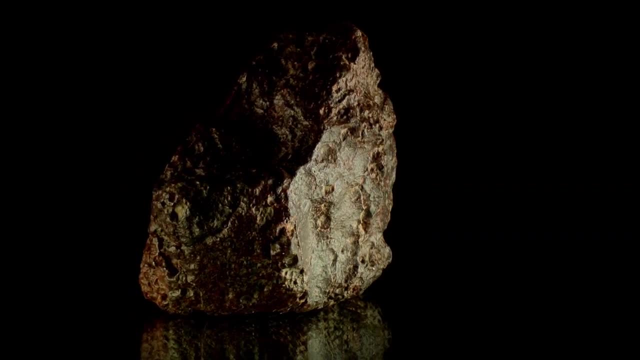 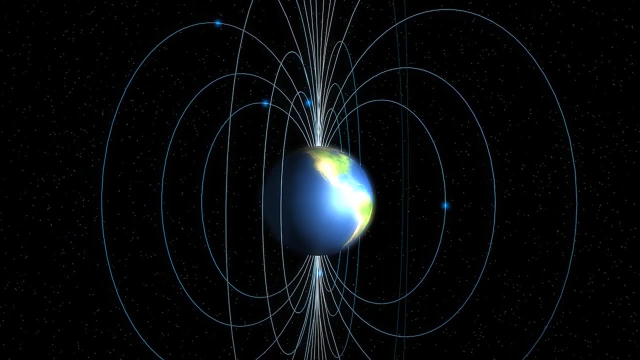 and copper. Also, metallic meteorites are thought to be representative of the core. Second thing: if Earth's core were not metal, the planet would not have a magnetic field. But we know a magnetic field exists around the Earth, A mechanism that could produce and sustain. 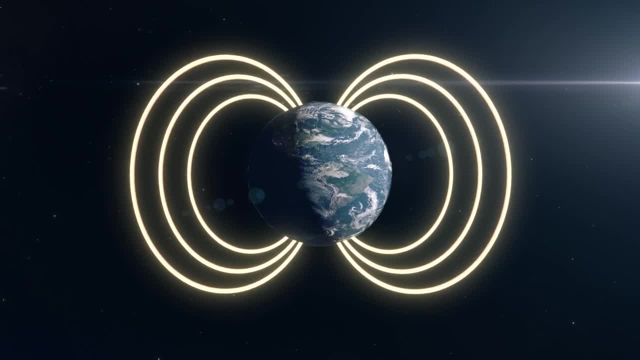 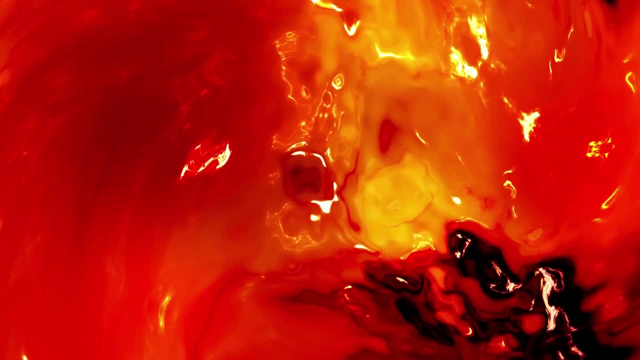 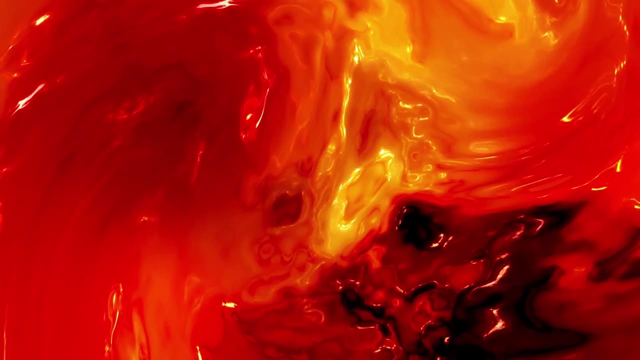 a magnetic field is the so-called dynamo mechanism. For this mechanism to act, the outer core of the planet must be liquid and the inner core must be solid. The strong magnetic field is caused by liquid outer core. Convection currents in the outer core are due to heat from the even hotter 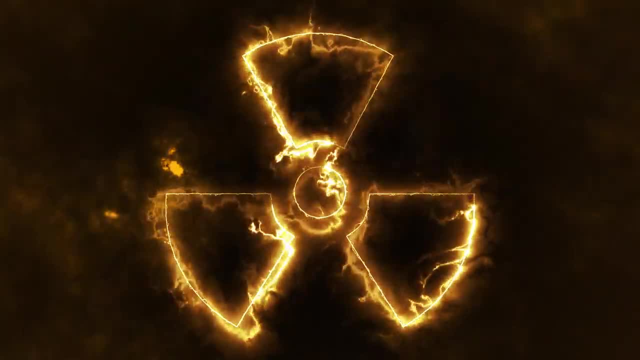 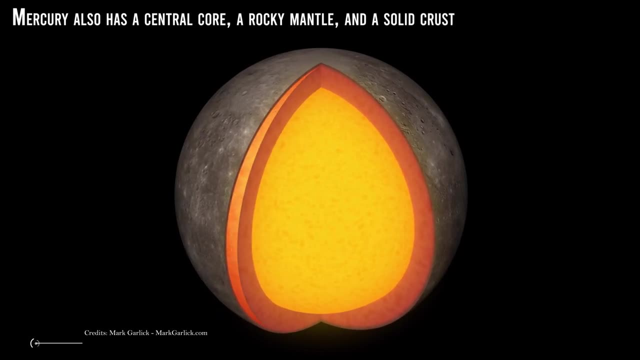 inner core. The heat that keeps the outer core from solidifying is produced by the breakdown of radioactive elements in the inner core. Speaking of mercury, it also has a central core, a rocky mantle and a solid crust, just like Earth. It's actually the second-densest planet. 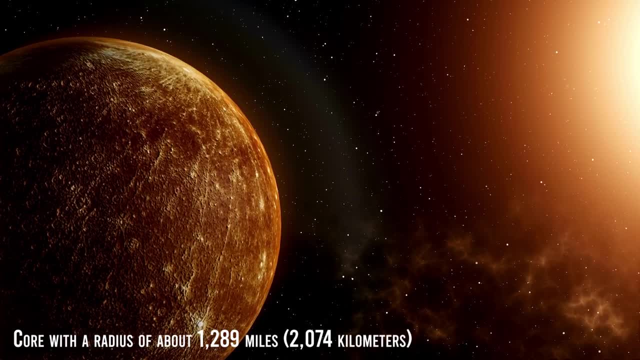 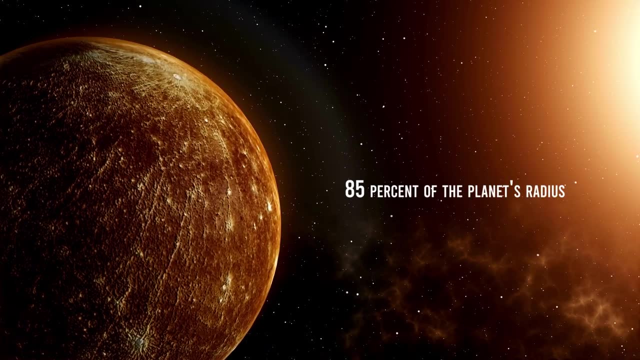 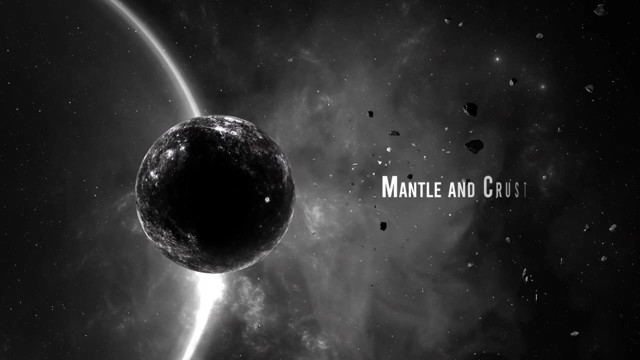 after Earth. It has a large metallic core with a radius of about 1,289 miles, about 85% of the planet's radius. There is evidence that it is partially molten or liquid Mercury's outer shell, comparable to Earth's outer shell called the mantle and crust. 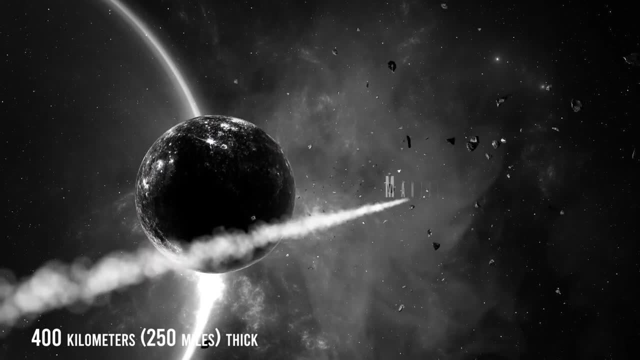 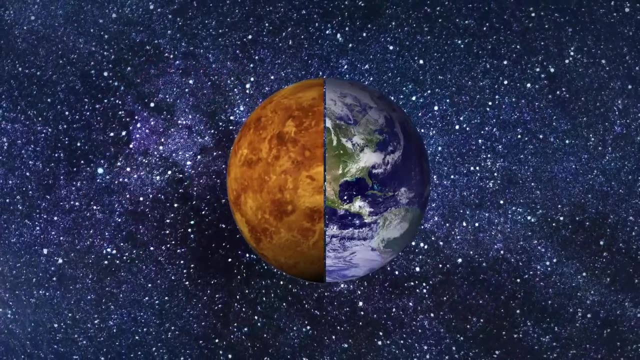 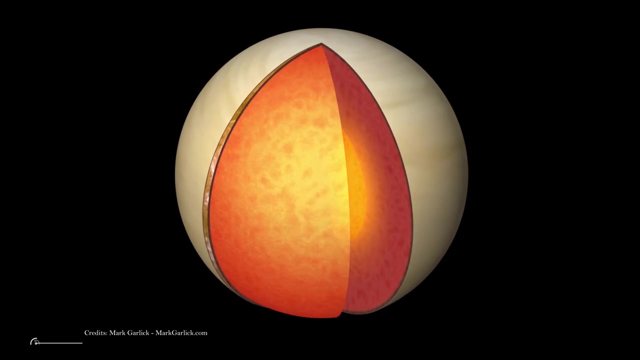 is only about 400 kilometers or 250 miles thick. What about Venus? Interestingly enough, if we could slice Venus and Earth in half, pole to pole, and place them side by side, they would look remarkably similar. They both have an iron core surrounded by a 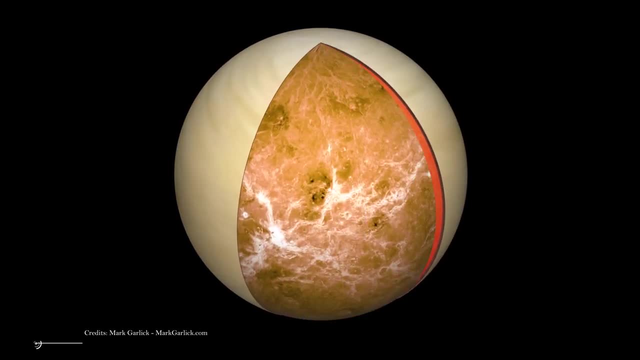 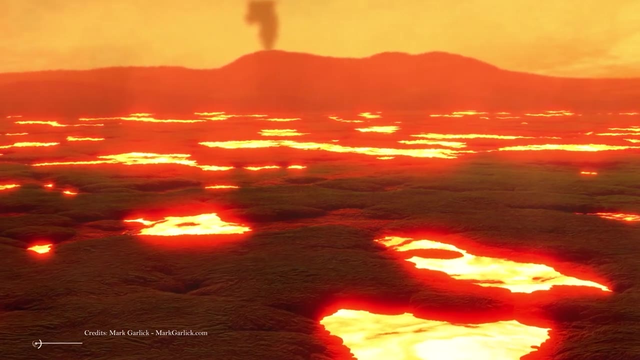 hot mantle, and they both have a crust which is a quite thin external layer. The crust is a sort of skin that changes form over time, causing volcanism. However, the two planets are also really different, For instance the plate tectonic's. 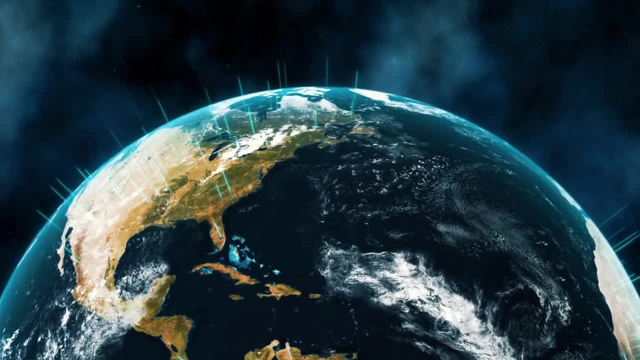 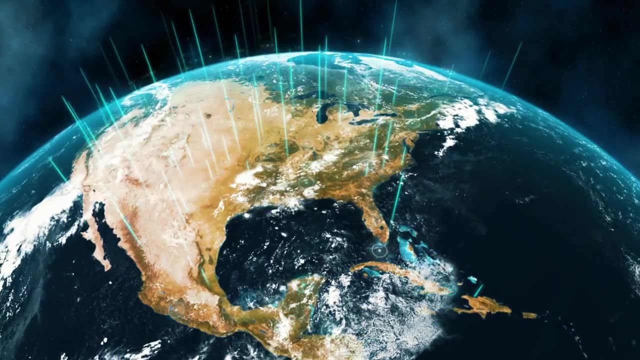 mechanism is active. It is the slow movement of continents over thousands and millions of years that reshapes the surface. This is not observed to be happening on Venus. If it did, it did in the early history of the planet. But we observe strong volcanic. 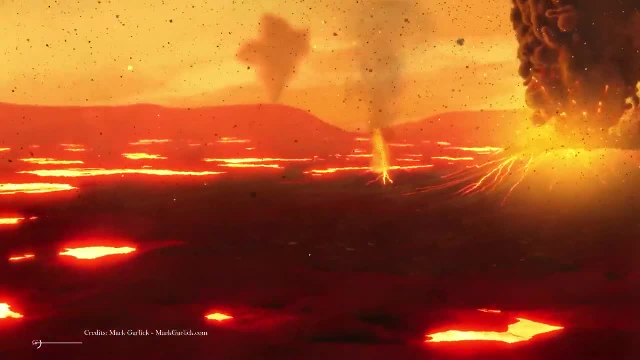 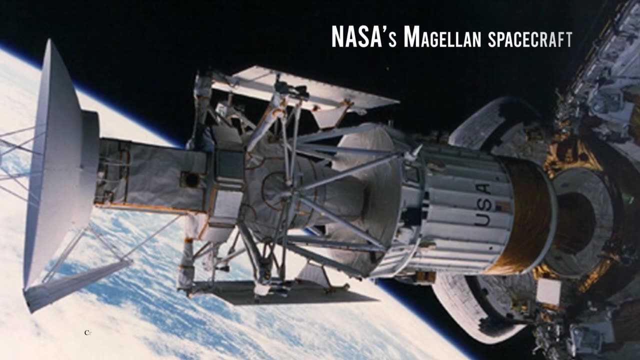 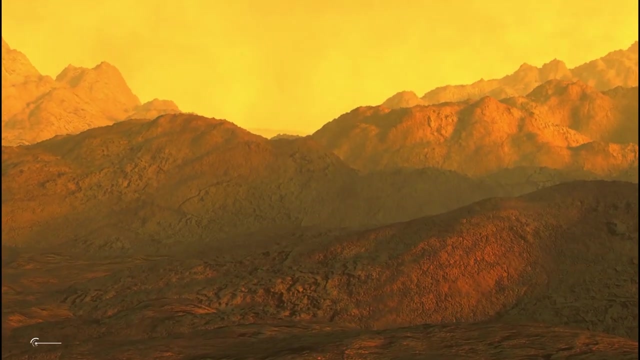 activity on Venus. This could be due to subduction, the sliding of one continental plate beneath another, which can also trigger volcanoes. NASA's Magellan spacecraft saw a land of extreme volcanism. The orbiter saw a relatively young surface, one recently reshaped in geologic. 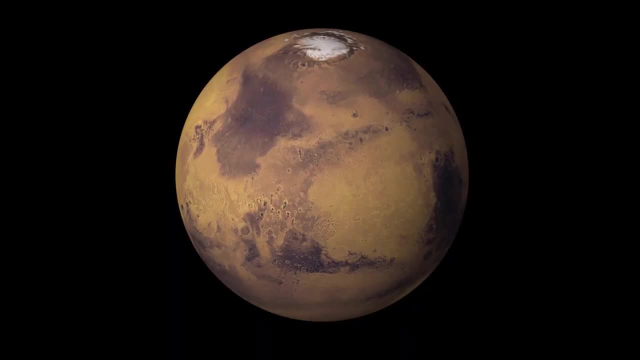 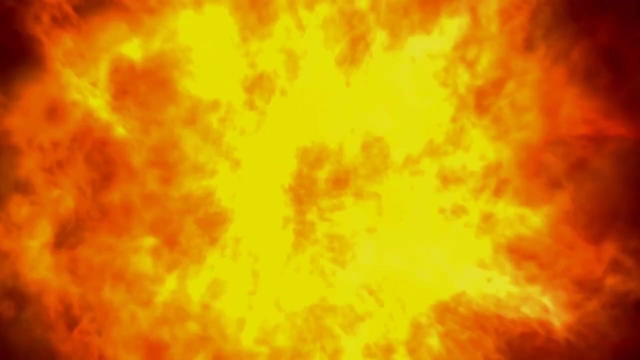 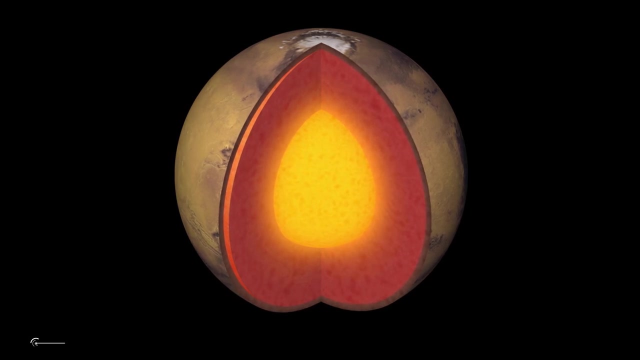 terms and chains of towering mountains. Last but not least, Mars has a dense core at its center, between 930 and 1,300 miles. It is made of iron, nickel and sulfur. Surrounding the core is a rocky mantle between 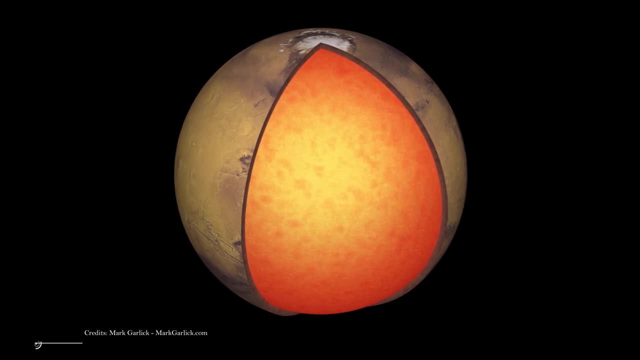 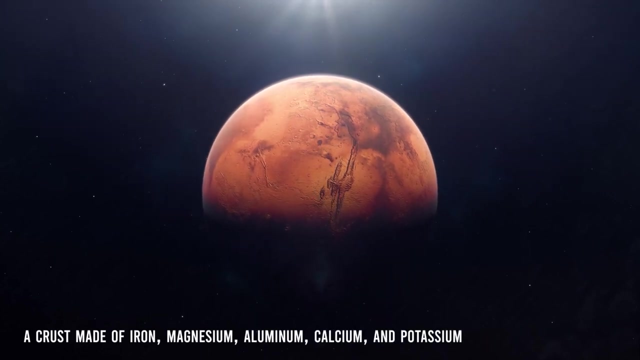 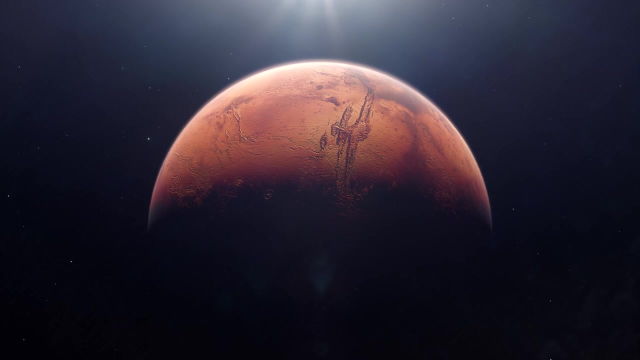 770 and 1,170 miles thick, and above that a crust made of iron, magnesium, aluminum, calcium and potassium. This crust is between 6 and 30 miles deep. The four gas giants in our solar system are Jupiter, Saturn, Uranus and Neptune. 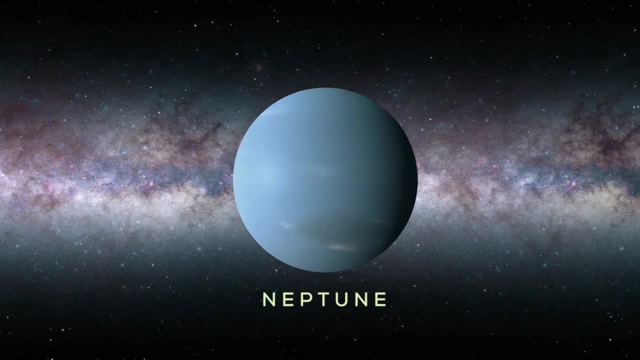 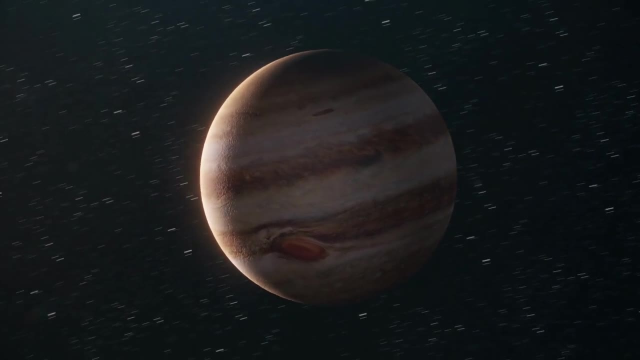 As we've already mentioned, they are also called the Jovian planets. A gas giant is a giant planet that is made of gas. They are different from rocky or terrestrial planets that are made of mostly rock. Unlike rocky planets, gas giants do not have a well-defined surface. 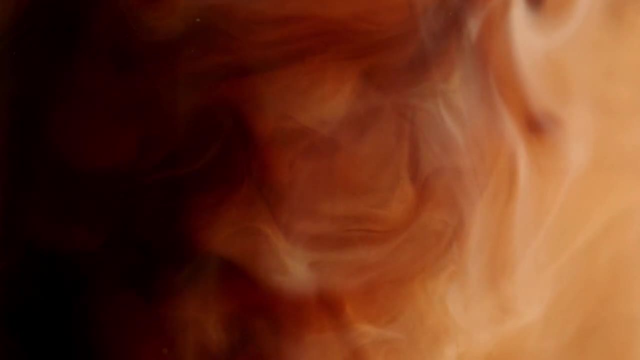 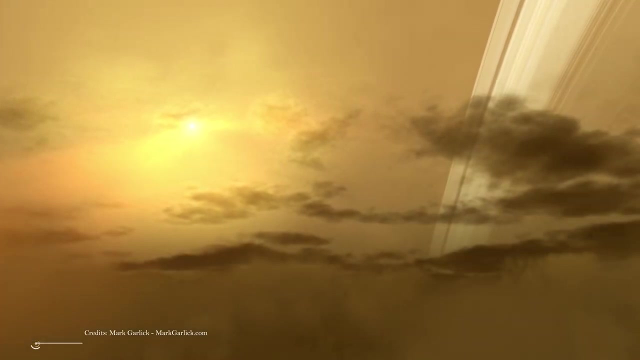 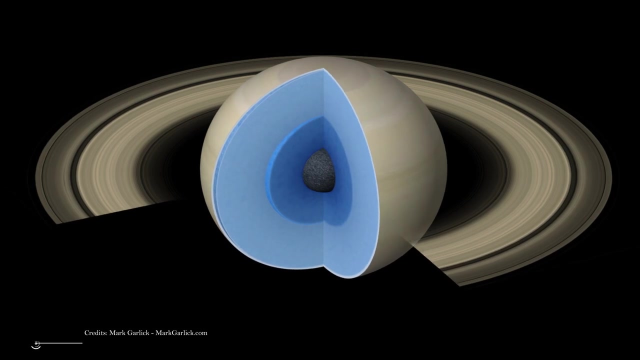 There is no clear boundary between where the atmosphere ends and the surface starts, and you can't walk or land on their surface. The gas giants have atmospheres that are mostly hydrogen and helium, the most common gases in the universe. Gas giants may have a rocky or metallic core, but the majority of their mass is in the form of gas. 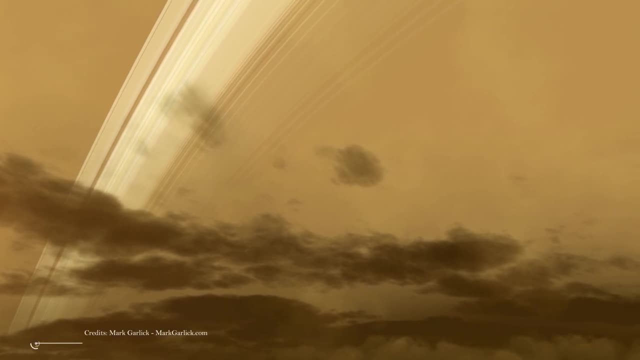 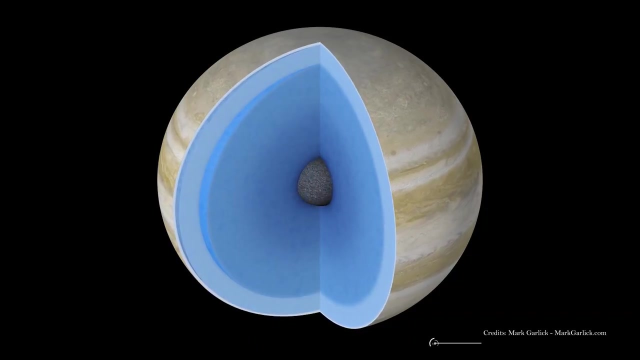 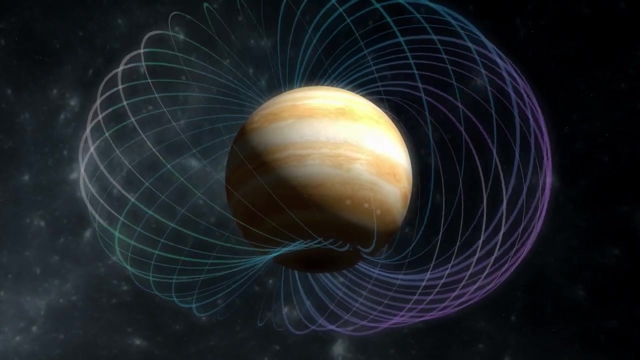 Since the pressure is really high. gas on these planets might also be compressed into a liquid state, just like mercury in a thermometer. Jupiter and Saturn probably have liquid metallic hydrogen interiors, which allows them to have a magnetic field, since liquid hydrogen conducts electricity. This is because the gas giant is a very high pressure element. Scientists 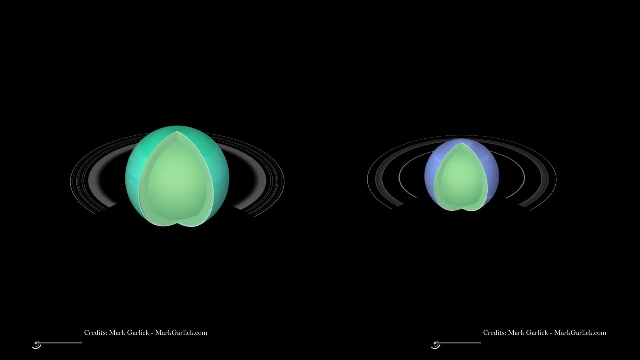 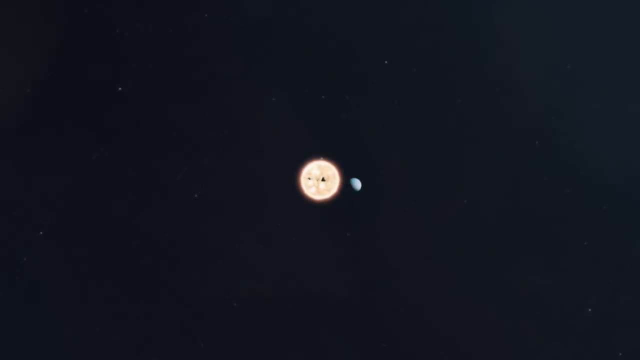 believe Uranus and Neptune have interiors that contain a mixture or layers of rock, water, methane and ammonia. So far we have given a brief description and overview of the composition of planets in our solar system. Now let's get to the point. Why are they different? 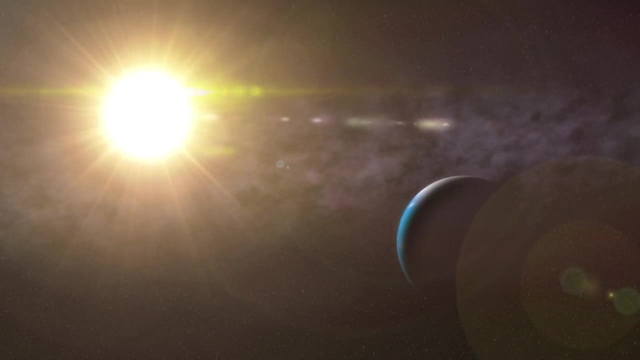 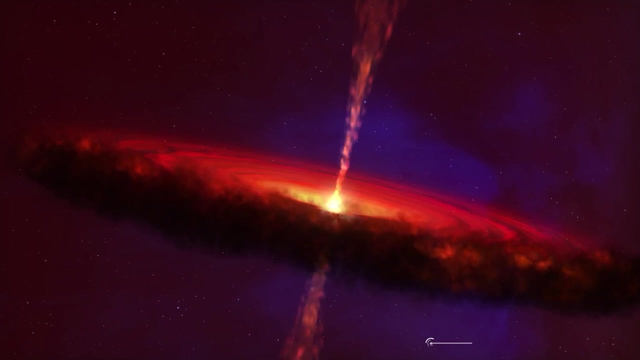 To understand why the rocky planets are closer to the sun, we must go back to when the solar system was young and the planets were still being born. The planets in our solar system are believed to have formed from the same spin. The planets in our solar system are believed to have formed from the. 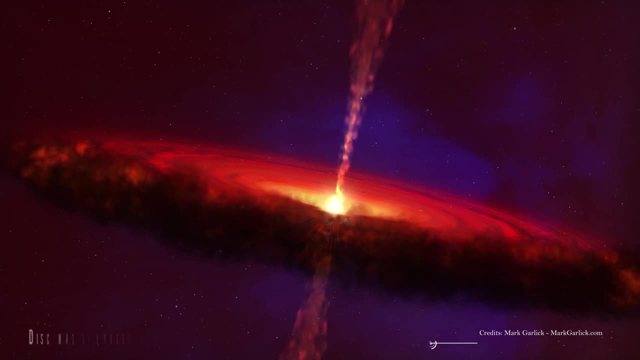 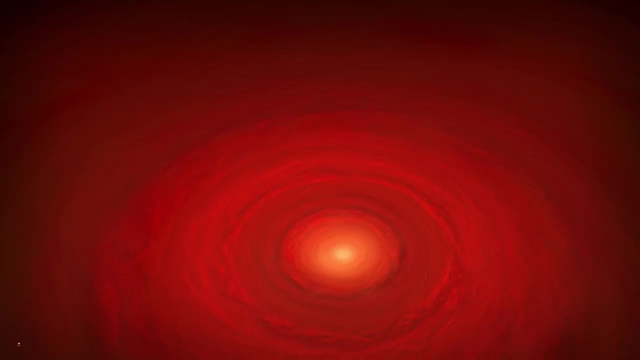 same spin. The planets in our solar system are believed to have formed from the same spin. The spin was formed by the spinning disc of dust that formed the sun. This disc was composed mainly of hydrogen and helium, but also had other elements in smaller proportions- Dust particles in the spinning disc began to clump together as gravity attracted them to each other. You have to think about it as a fight. During this period, clumps of matter were trying to grow as big as they could in order to overcome the others in size, thus being the 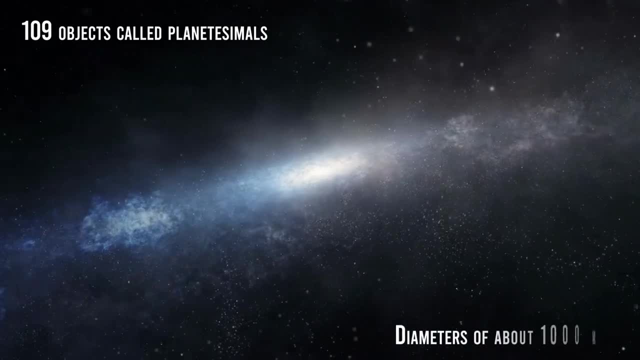 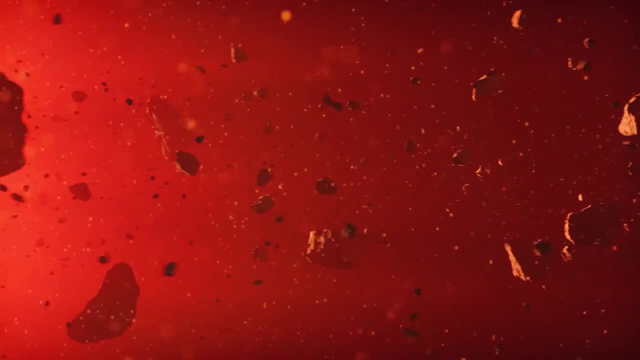 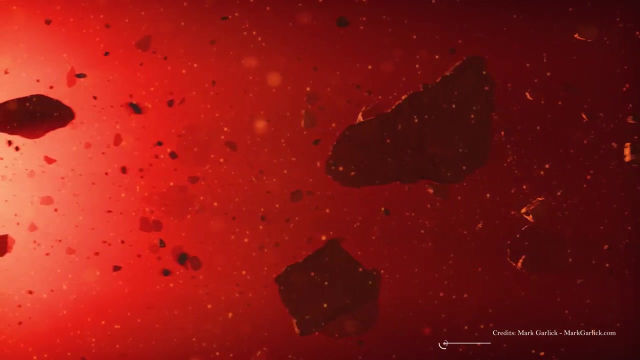 dominating objects in the disk. Over a few million years, many of these chunks had merged together, merged together and there were about 109 objects called planetesimals, with diameters of about 1000 meters. Over time, the planetesimals continued to collide and join together, attracted by gravity. 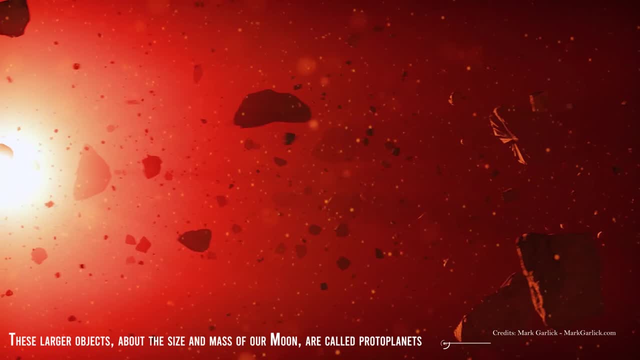 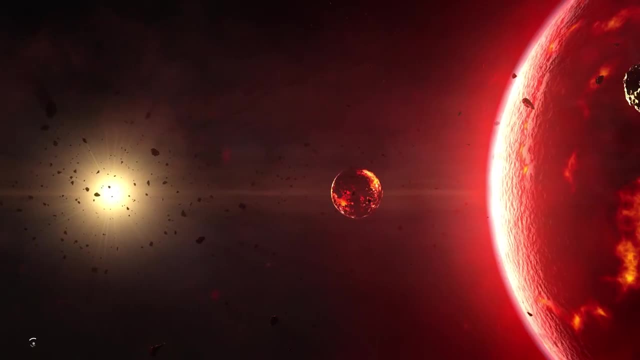 These larger objects about the size and mass of our Moon are called protoplanets. The accumulation of material to form planets in this way is called accretion. The solar system in its youth was very chaotic. All the planets and even our own Sun. 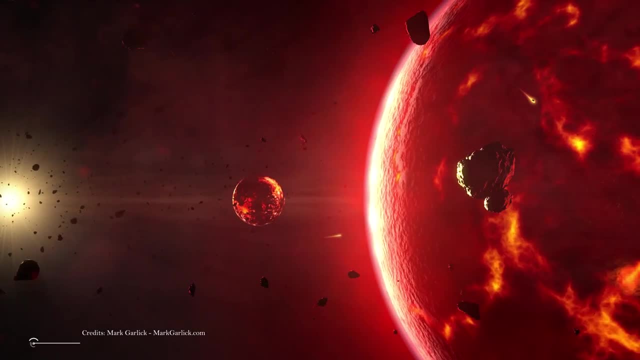 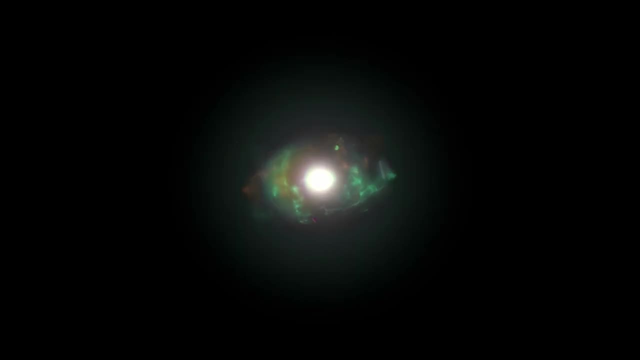 were in exotic and excited states. For example, the Earth was basically a ball of lava a long time past before it cooled down. In the early solar system there were many collisions and explosions and heat waves passing between them Once upon a time. 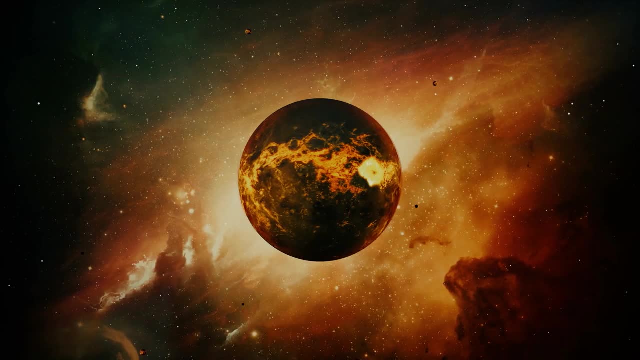 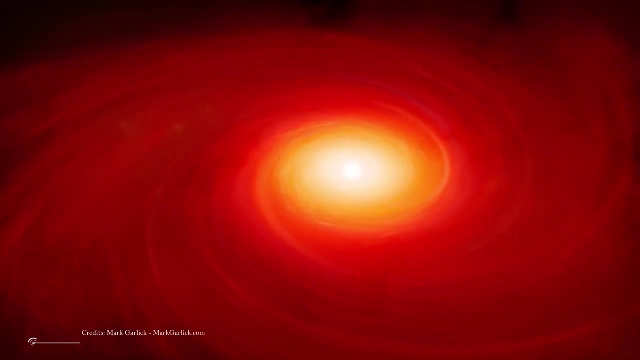 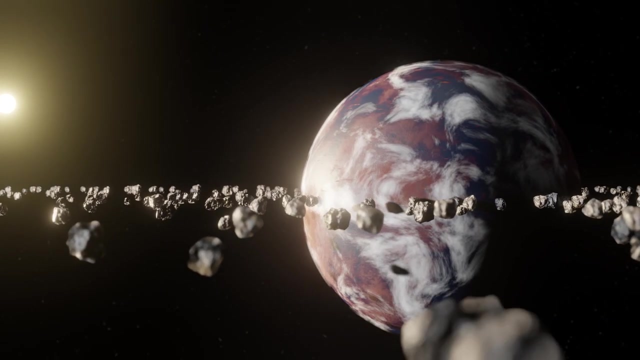 the rocky planets we see now also had huge gaseous layers around them, just like the gas giants and ice giants. However, during its angry young years, the Sun let out huge streams of energy and matter into the solar system. The rocky planets, being the closest to the sun, took the full force of these streams. This made the 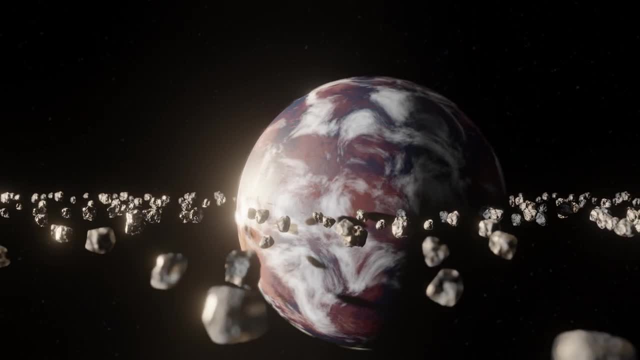 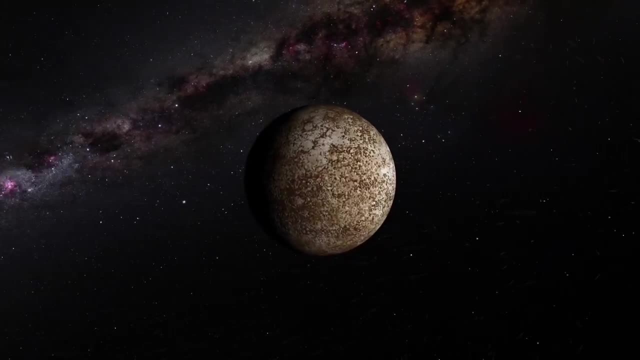 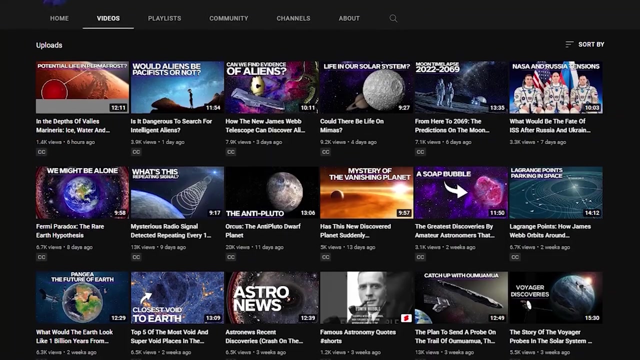 gases of these planets part ways with them, leaving just the rocky part behind, which went on to become the terrestrial planets. The remaining four planets were too far from the sun to experience these streams, so they stayed relatively unaffected and formed the gas and ice giants of today. If you're still watching, it means you really liked this video. 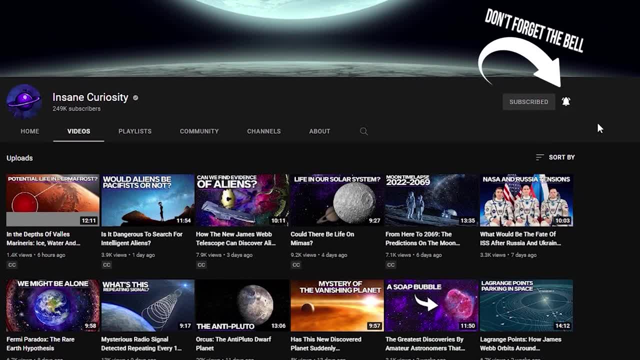 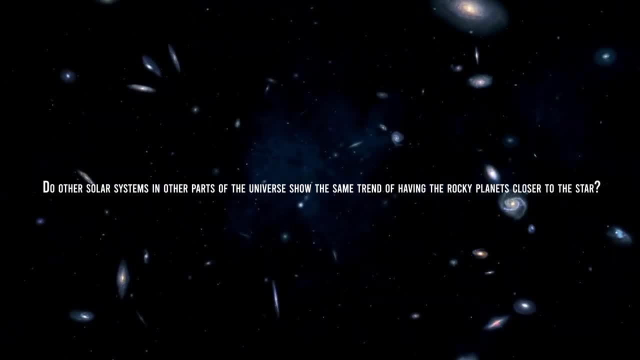 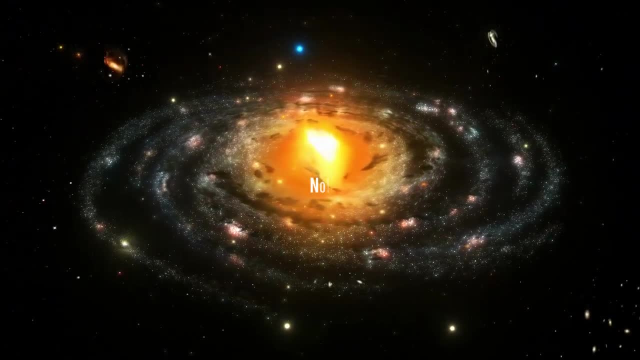 Why don't you subscribe and press the notification bell? So is this a pattern that we see everywhere? Do other solar systems in other parts of the universe show the same trend of having the rocky planets closer to the star, while the massive gas giants are quite far away? The answer is no. Scientists have found many solar 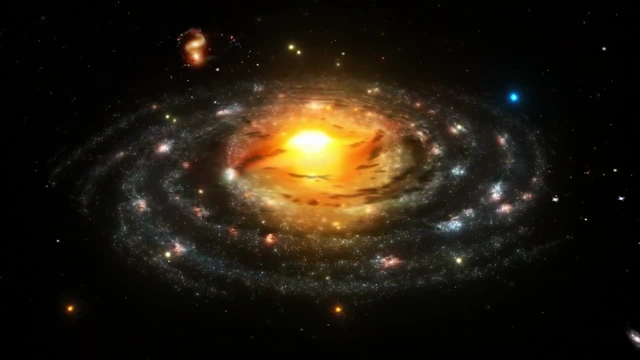 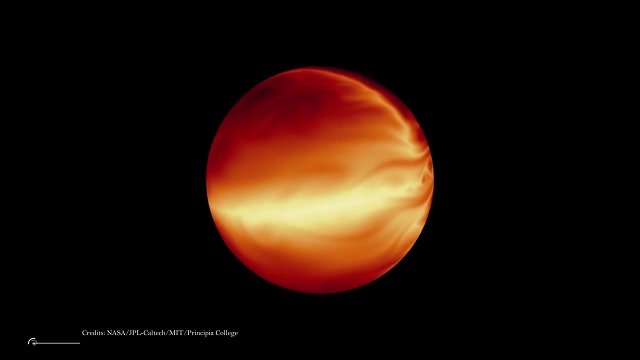 systems in which gaseous planets, many of which are even more massive than the gas giants of our solar system, are the ones closest to their stars. For instance, they found a lot of hot Jupiters. Hot Jupiters are Jupiter-like planets orbiting really close.